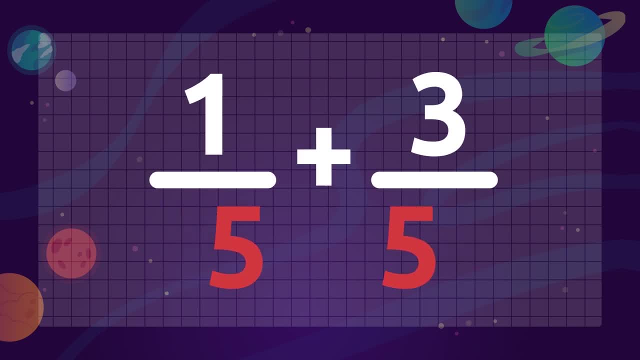 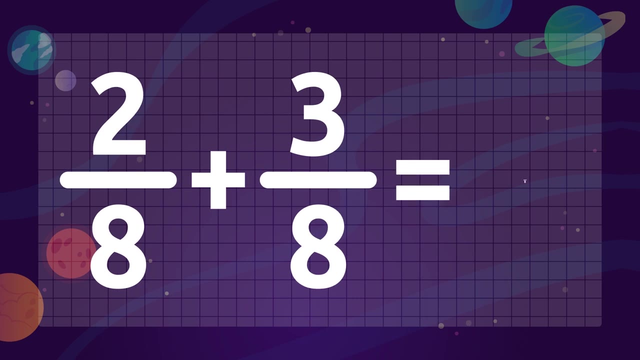 To add fractions with the same denominator, we leave the common denominator and add the numerators. It's very simple. Let's see an example. To add 2 over 8 plus 3 over 8, we leave the common denominator, in this case it's number 8, and we add the numerators, that is 2 plus 3, which equals 5. This result, number 5, will be the numerator. 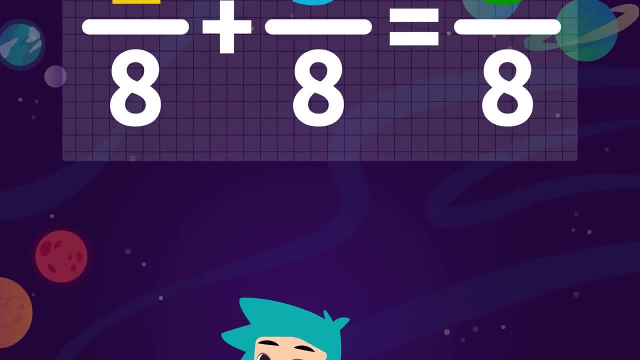 The result is 5 over 8. Are you up for a challenge to practice a bit more? 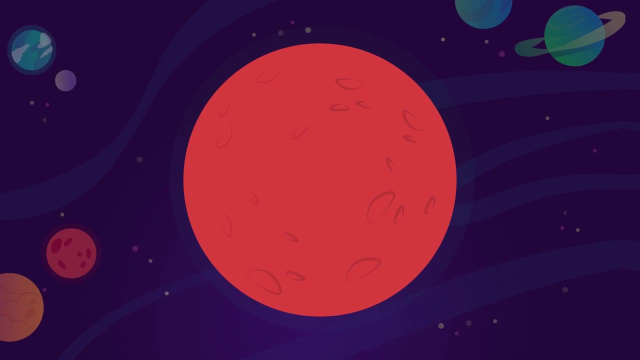 In the Smile and Learn universe, there's a planet called Smileython. This planet is divided into 8 equal parts. Two eighths of the planet are occupied by friendly aliens and the remaining three eighths by grumpy aliens. What fraction would represent the overall number of land occupied by all the aliens on the planet? 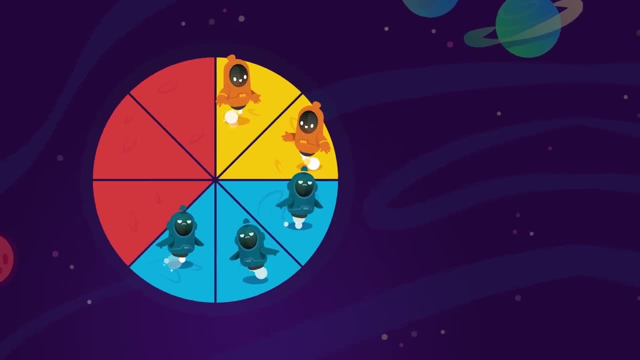 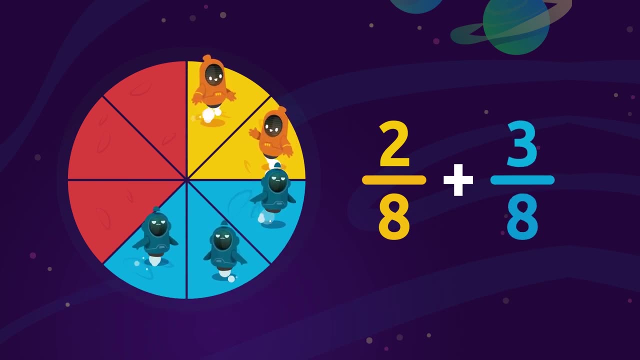 To find out, we'll need to add the fractions. Two over eight plus three over eight. Do you remember how to do this math operation? Remember that the result would have to be the same denominator. In this case, it would be the number 8. And now to calculate the numerator, we'll add the numerators 2 and 3, which equals 5. The result will be that 5 eighths of the land 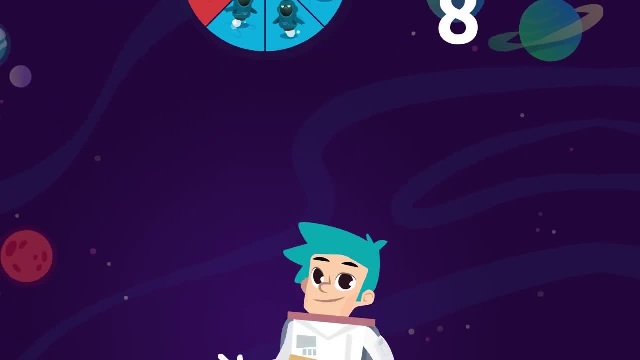 are occupied by aliens. Will you help me figure out something else? Let's learn a little. Let's learn the math. Learnython, 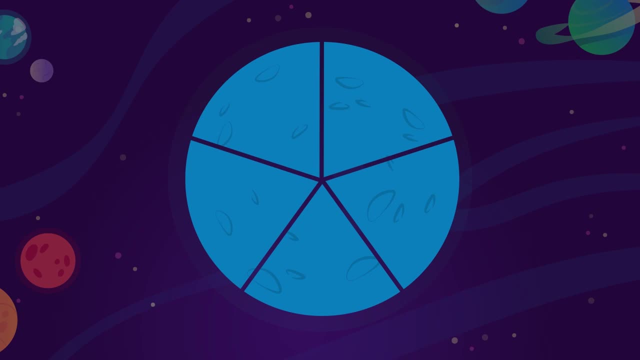 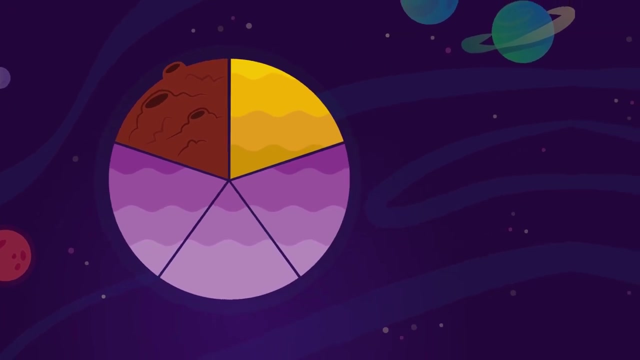 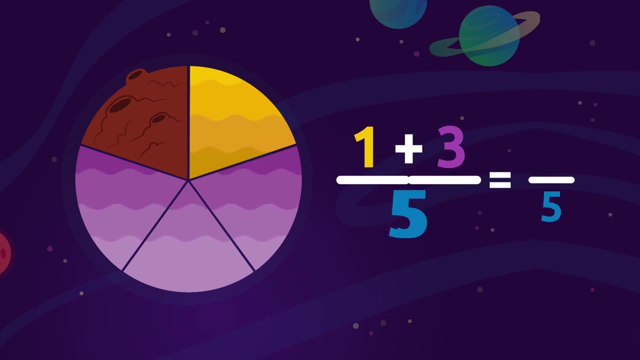 our neighboring planet, is divided into five equal parts. There is yellow water on one-fifth of the planet, purple water on three-fifths of the planet, and volcanic soil on one-fifth of the planet. How much of the land on Planet Learnython is covered with water? To find out, we'll need to add the fractions 1 over 5 plus 3 over 5. First, in the result, we'll leave the 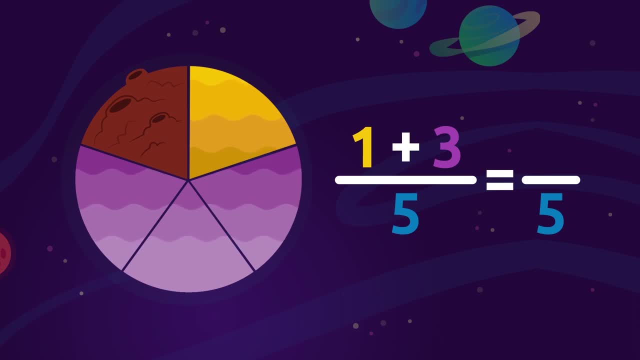 common denominator, and then we'll add the numerators 1 plus 3, which equals 4. The result will be that four-fifths of the land of the planet are covered with water. Thank you for helping me! 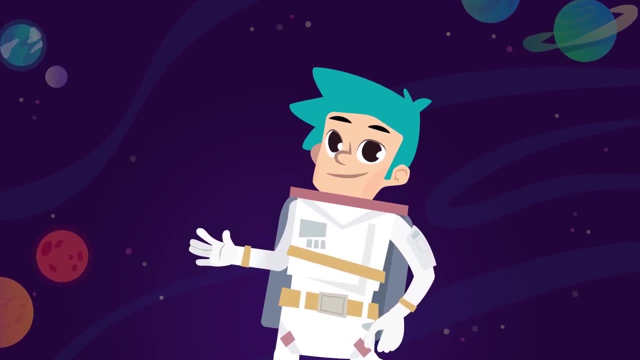 Now you know how to add fractions with the same denominator. Little by little, you're getting better at it! 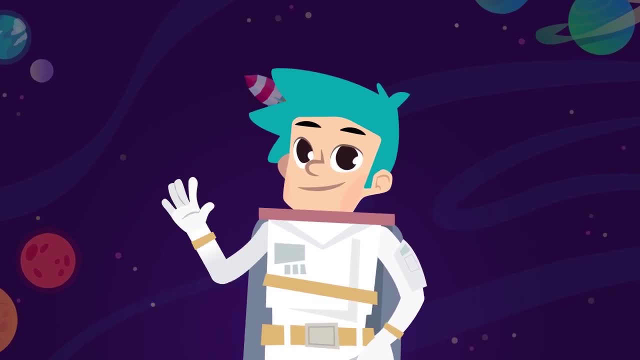 You're going to become math experts! Keep up the good work! See you around! 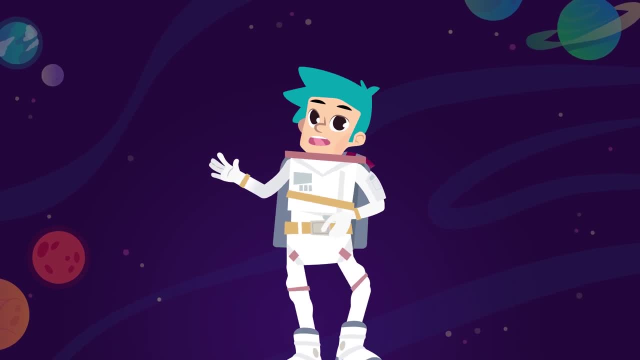 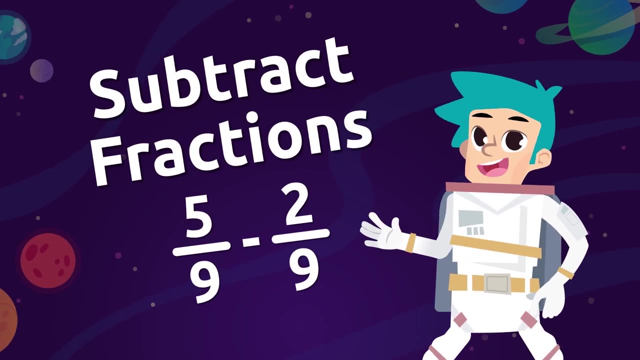 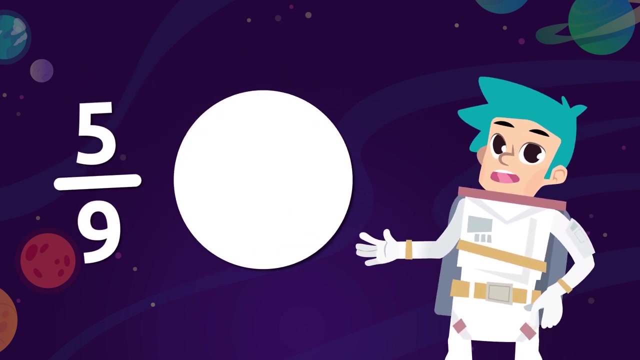 Hello again, math friends! We're going to continue learning about fractions. Today, we're going to learn how to subtract fractions with the same denominator. Do you remember what a fraction is? A fraction is a number which indicates the division of a whole number in equal parts. 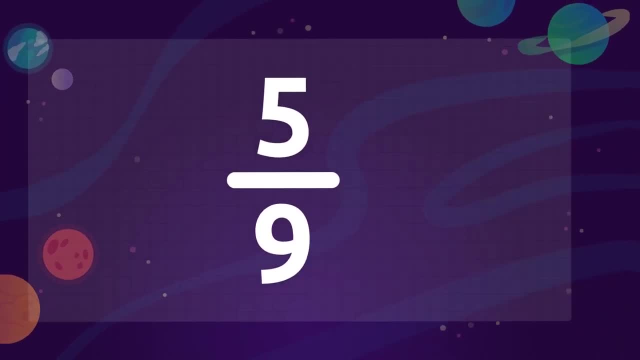 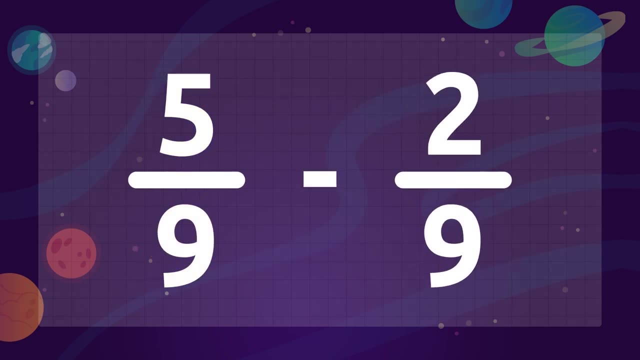 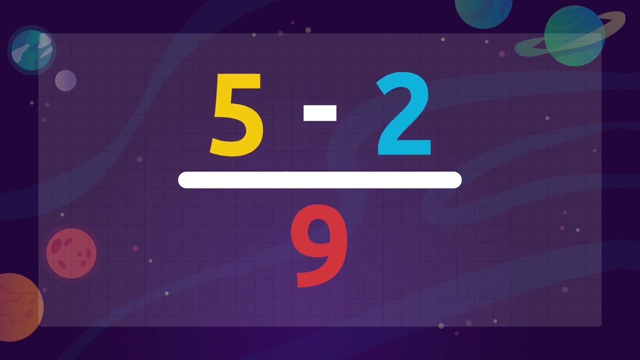 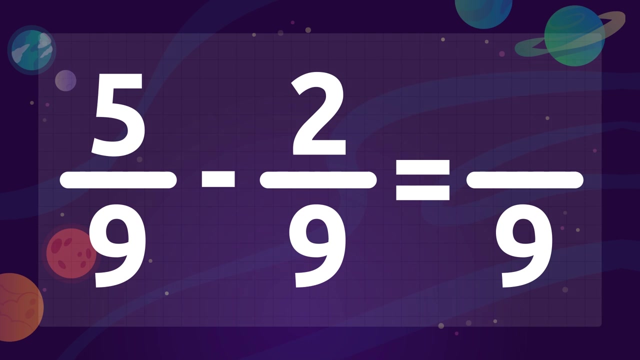 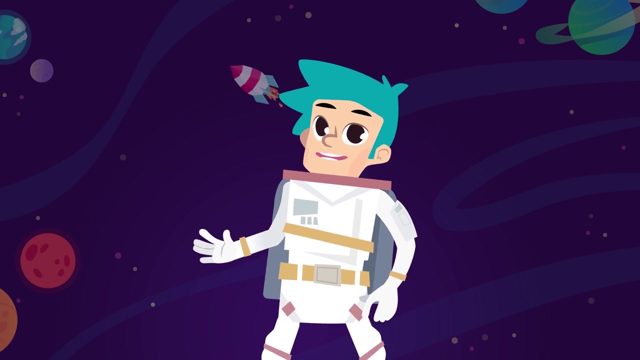 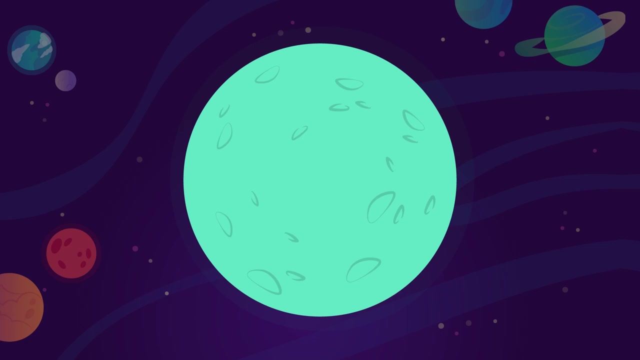 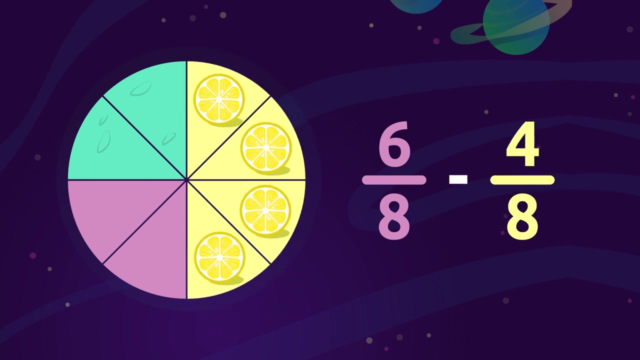 First, let's remember which are the parts of a fraction. This is the numerator, and this number is the denominator. To subtract fractions with the same denominator, we leave the common denominator and only subtract the numerators. It's very simple. Let's see an example. We need to solve this math problem. Five-ninths minus two-ninths. The denominator, which is the numerator, stays the same. In this case, it's the number nine. Now we subtract the numerators. That is, five minus two, which equals three, which will be the numerator in the answer. The result of this math problem will be three-ninths. Are you up for a challenge to practice a bit more? In the Smile and Learn universe, there's a planet called Smileython! The planet is divided into eight equal parts. In six of these eight fields, they grow apple trees and lemon trees. If four of the eight fields are planted with lemon trees, how many fields are planted with apple trees? To find out, we'll have to subtract fractions. We need to subtract the total number of fields planted with fruit trees from the number of fields planted with lemon trees to find out how many apple tree fields there are, meaning six-eighths minus four-eighths. Do you remember how to do this math operation? Remember that we should put the same denominator in our answer. In this case, number eight. Now, to calculate the numerator, 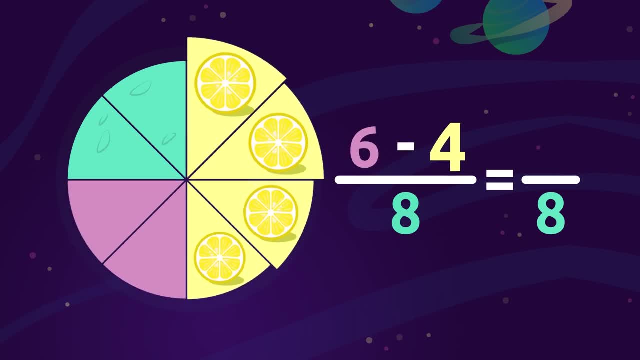 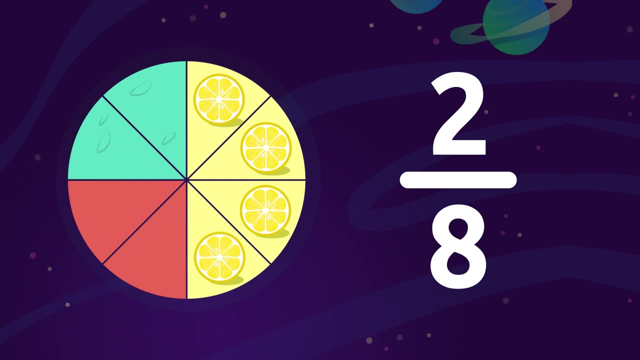 we subtract the numerator's six minus four, which equals two. The result is that two of the eight fields are planted with apple trees. That is two-eighths. 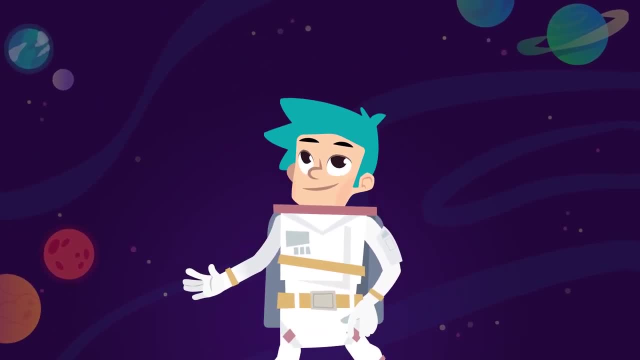 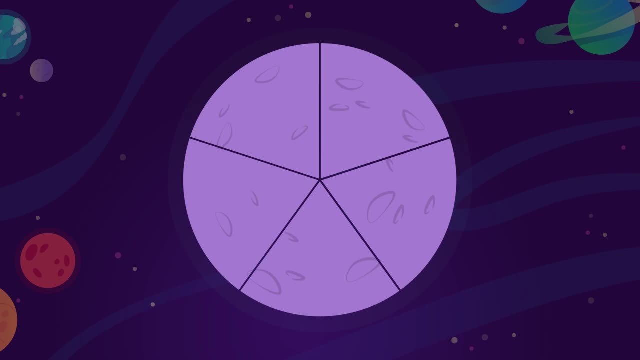 Will you help me figure out something else? Planet Learnturn is divided into five equal parts. On this planet, there are wooded areas and areas with houses. If they built houses